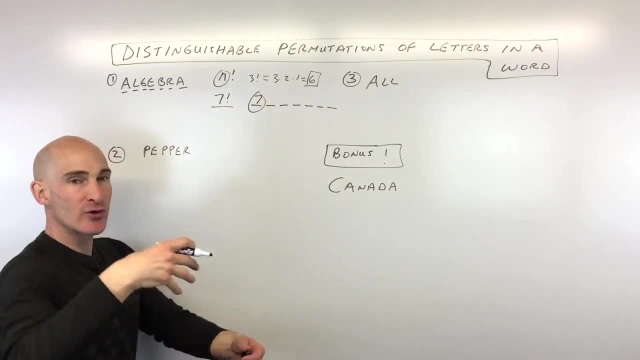 See 1,, 2,, 3, 4,, 5, 6, 7.. There's going to be 7 choices, like if you were to reach into a hat. 7 different, you know choices for picking out that first letter. 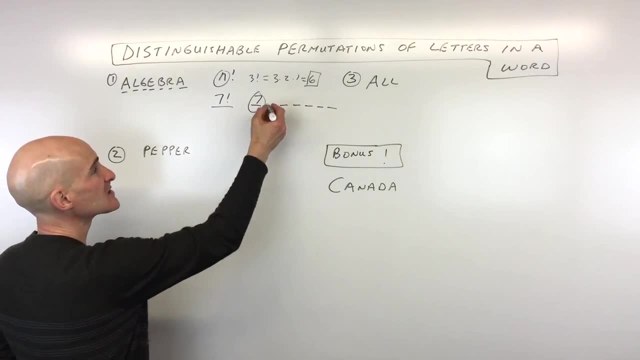 Once you pick out that first letter, how many are there left to choose for the next letter? in the word, There's going to be 6, right, And then 5, and then 4, and then 3, and 2, and 1.. 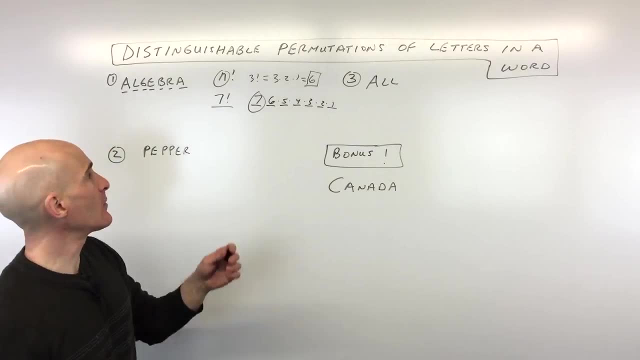 That's the same as what I've written here. 7, factorial, So that's another way to think about it. The only problem is, though, is you see how it says distinguishable? That means that you know they look like they're different. 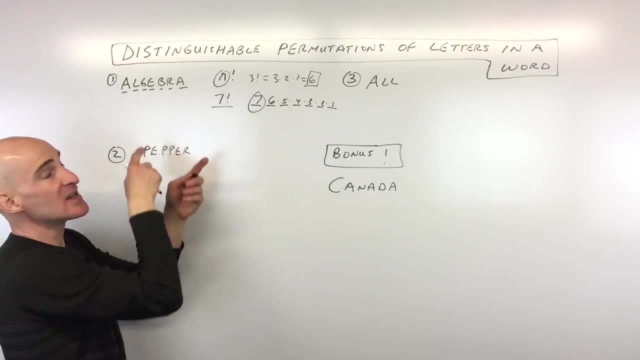 If I just move this A over here to this A over here, like switch these 2, As it would still look like the word algebra. So what we have to do is we have to see if there's any repeated letters Here. you can see there's 2 As that are repeated. 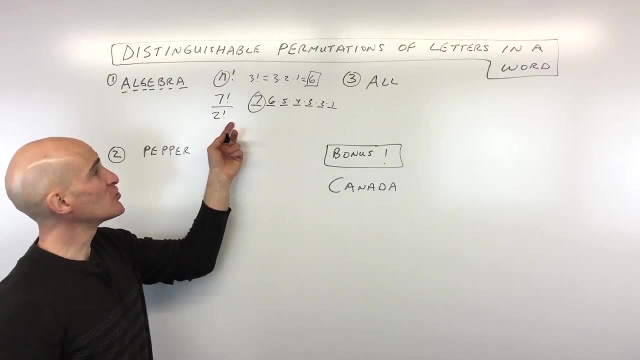 So I'm going to do that, So I'm going to do that, So I'm going to do that. So I'm going to divide by 2 factorial. 2 factorial is just 2 times 1.. That means there's 2 different ways of arranging these, As okay, you know, such that, you know, it wouldn't really look like a different word. 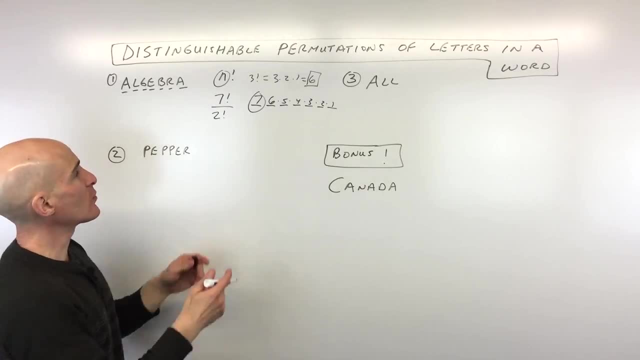 So we have to divide out those multiplicities, if you will. So here we're just going to go ahead and simplify. So 7 factorial- we've already written that out- Divided by 2 factorial, which is 2 times 1.. 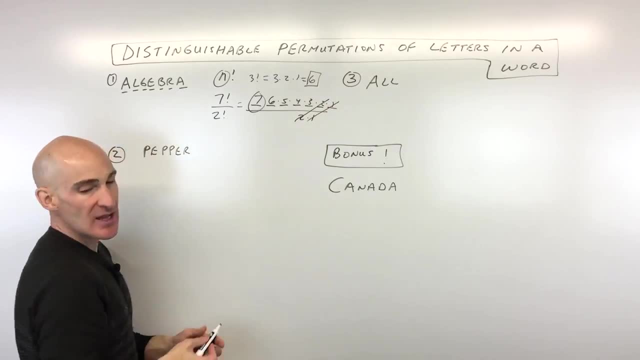 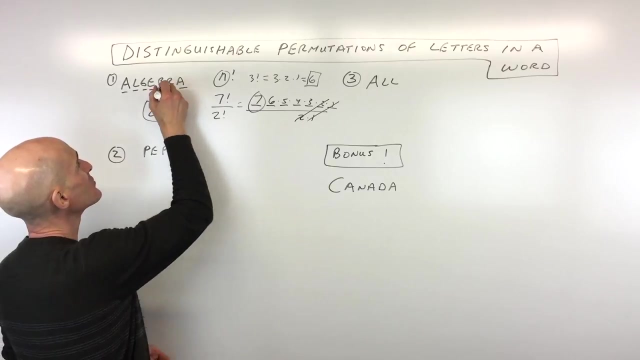 And you can see the 2 and the 1, those are going to cancel. So we really just have to multiply 7 times 6 times 5 times 4 times 3.. So let's go ahead and do that. Let's see times 5 times 4 times 3, which is 2,520 different ways of using all the letters in algebra to make a different, distinguishable permutation, which is like an ordering of those letters, right. 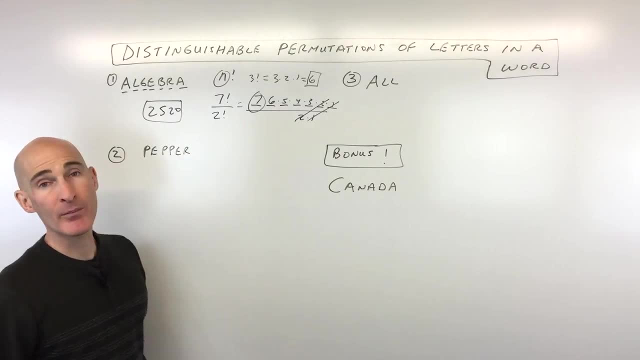 So let's go ahead and do number 2.. See if you can do this one. We've got the word pepper, okay, So pepper, let's see. this one has 6 letters. So that means there's going to be 6 factorial ways of arranging 6 of those you know letters. 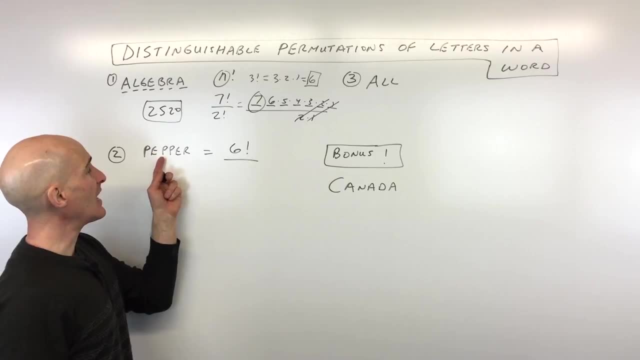 The only issue is we've got 3.. We've got 3 P's and 2 E's, right? So we have to divide out those multiplicities. We're dividing out the 3 factorial for the P's and we're dividing out the 2 factorial, that's for the E's.